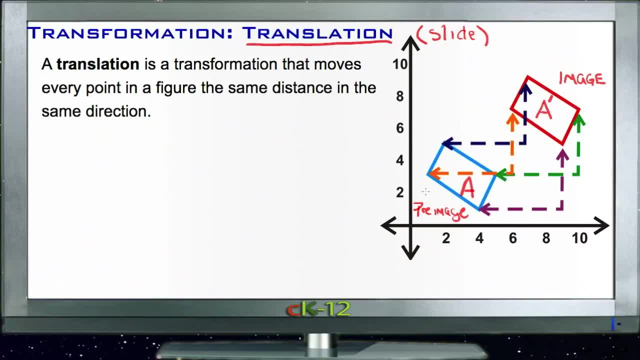 the same thing. It's just another way to notate it, To identify what's happened to a figure. specifically, with a slide we talk about what happens to any given point on the figure and its corresponding point on the image afterward. So from the preimage to the image, If for. 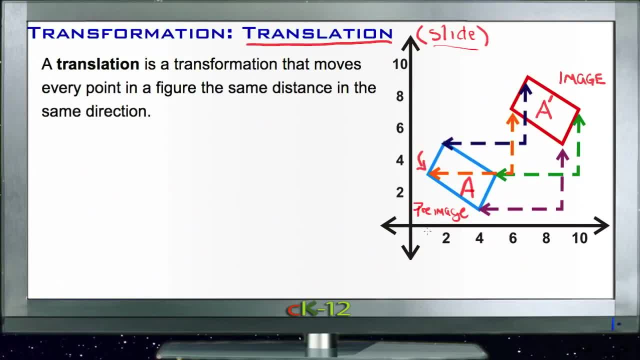 instance, we start with this location right here. This location looks like 1, 3.. So if this point right here is at 1, 3 on our preimage, and then the corresponding point is over here at 6, 7.. 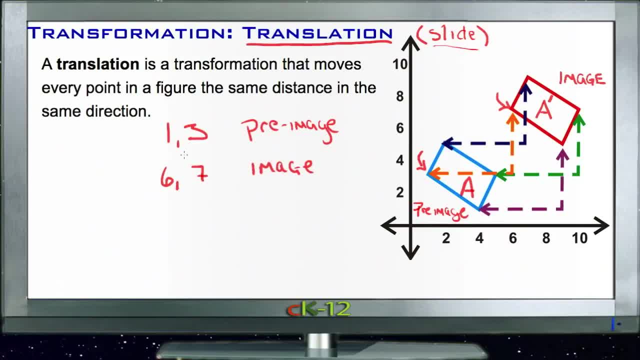 On the image then to get from one to the other. our x- remember our coordinates are x, comma, y, right. Our x change is going from 1 to 6, so it's a positive 5.. And our y change is a positive 3 to 7, positive 4.. So what we would say is that any location on our first 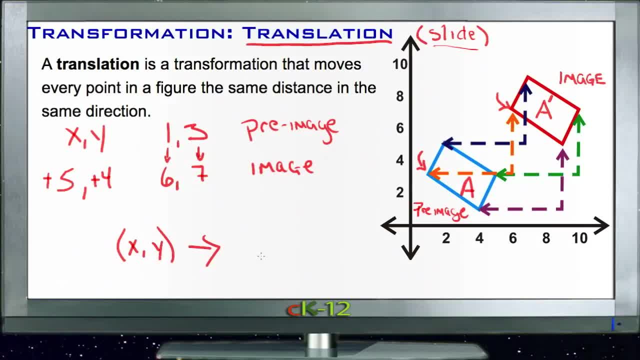 image translates to x comma y right, x plus 5 and y plus 4 on our new image. So obviously we can see we went up by 5 and up by 4 from our preimage to our image. so we can do that with any other point on the preimage. 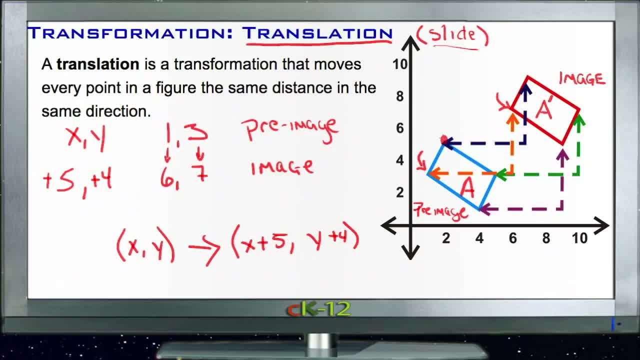 to get it to the same point on the image- Let's take a look at this one up here- say: This point here is 2, 5.. So if we put it through our little process, we start with 2 comma 5,. 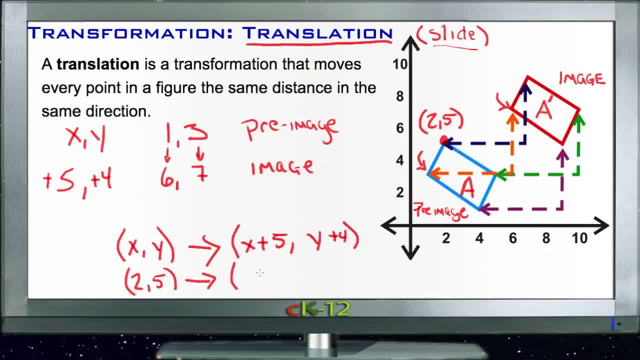 so we translate that point 2 plus 5 is 7, and 5 plus 4 is 9.. So the corresponding point should be at 7.. And it is, and 9.. And it is. This point up here is 7, 9.. 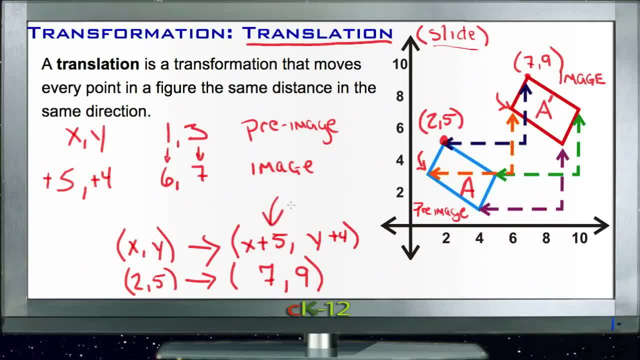 So that's the process: We look to see what we do to each x coordinate and what we do to each y coordinate in order to see what happens with the original preimage, to get into the location of the new image, and the image should be exactly the same in appearance. 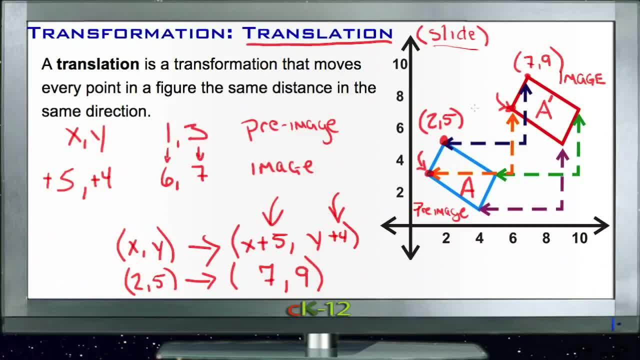 as the pre-image, if we're translating it or sliding it, because we're not going to change the way it looks, we're just going to change its location.